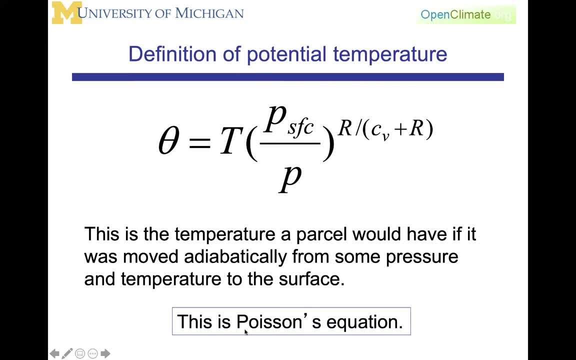 the definition of potential temperature, which is Poisson's equation. The potential temperature is the temperature a parcel would have if you moved it adiabatically from some pressure and temperature to the surface of the Earth. That definition goes back to our consideration of potential temperature. But if we move it adiabatically then we are saying that we 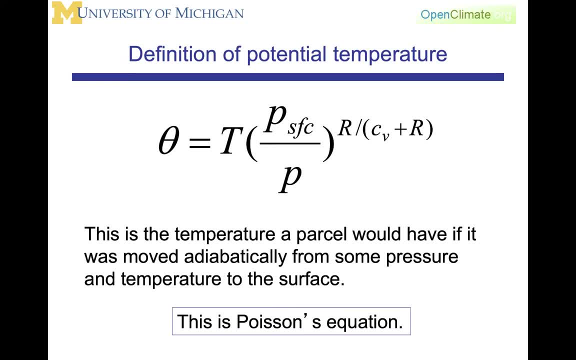 have no J-term in that equation. So there's no radiation, there's no thermal conductivity, there is no heat coming into or going out of the system. Hence the changes in temperature are going to be related to the equation of state and the relationship between pressure. 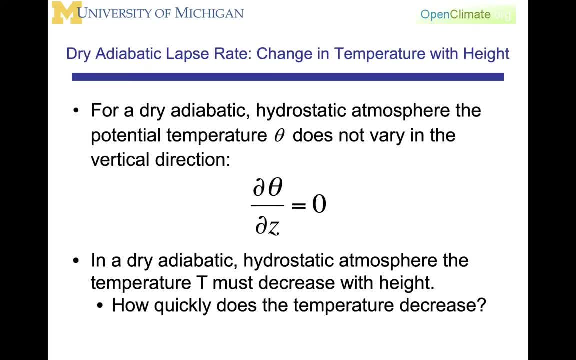 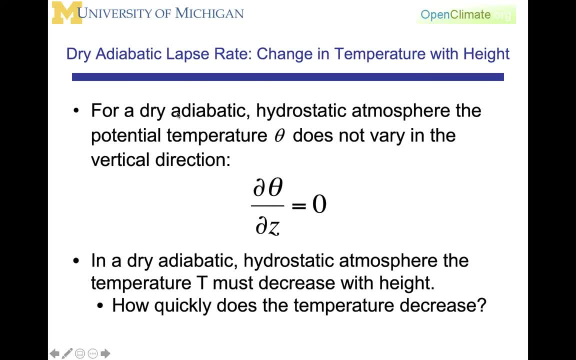 the atmosphere explicitly to be dry. Hence we will be talking about the dry adiabatic lapse rate and the dry adiabatic lapse rate. in a hydrostatic atmosphere. The potential temperature theta does not vary in the vertical direction. There's a lot packed into that for hydrostatic atmosphere, so that 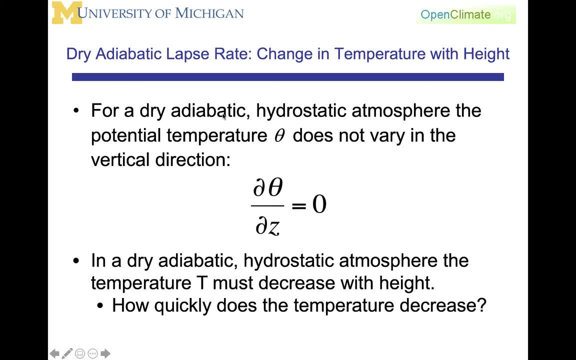 dp dz is equal to minus rho g, and if it's dry and there is no heat coming into or out of the system, then d theta dz is equal to zero. That means that in hydrostatic atmosphere the temperature t must decrease with height, because the density and the pressure are both decreasing with height. 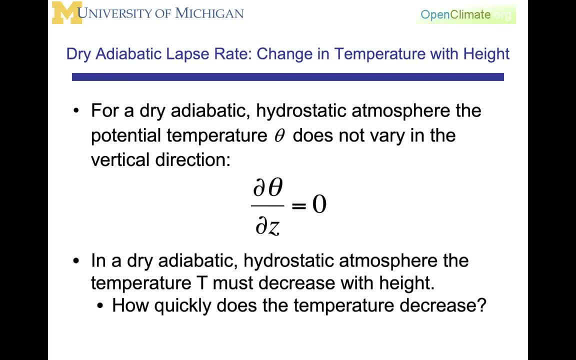 This is again similar to one of the homework problems That you did about what would be the temperature at the top of an atmosphere at constant density, and there are a number of ways you can play with the hydrostatic equation to try to understand how temperature pressure and density would vary under these idealized and thoroughly unrealistic. 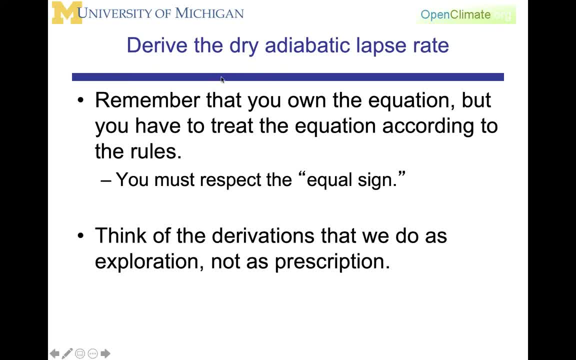 situations. What we want to do is to derive the dry adiabatic lapse rate. Again, I want to remind you that you own the equation And if you own the equation, you do have to treat the equation according to a set of rules, but you can manipulate it however you want to. 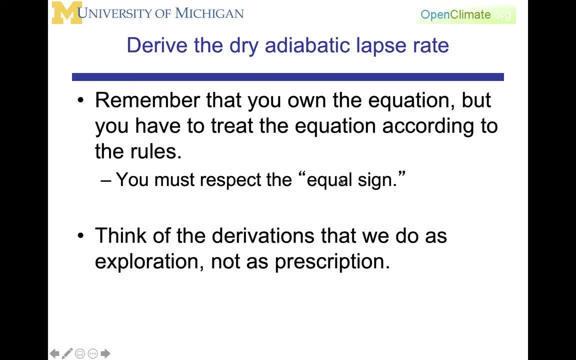 One of the rules that you must keep in mind is the equal sign, which means that if you do something to one side of the equation, you have to do it to the other side to maintain that equality. And again I'm going to say: think of derivations that we do as exploration. They're not prescribed, We don't have to do that. 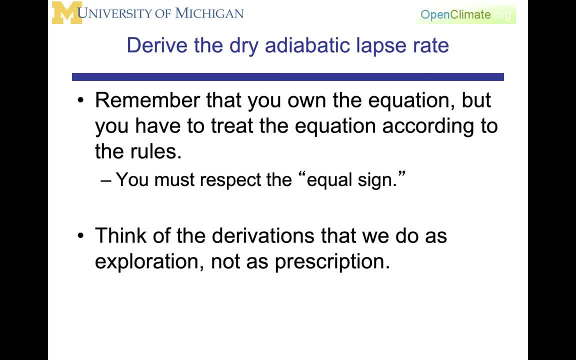 They're not prescribed, We don't have to do that, We don't have to do that, We don't have to do that. We don't have any hard and fast rule, though we do have well more than a century of, maybe, best practices to get results that we know are useful. 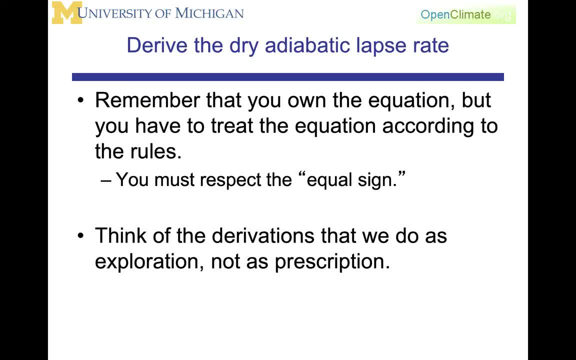 But even with more than a hundred years at this game, occasionally you can play with the equations and think about something you want to investigate and come up with a new method of analysis, a new approach. It's especially true if you bring in other fields, such as, perhaps, statistics. 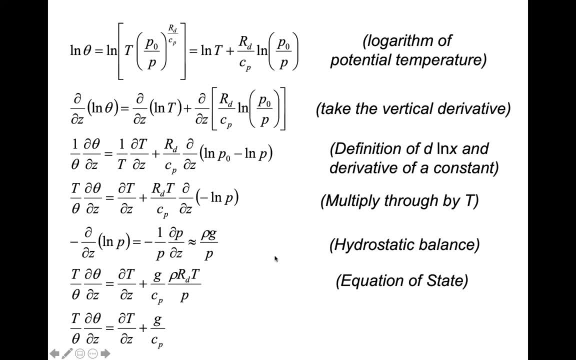 So all I'm going to do here I'm going to tell you about Cambridge equations. The home data is from this course- logarithm are doing exponentials in the vertical. what we're doing is we're really recognizing the exponential decrease of pressure with height, So we're taking advantage of that really very. 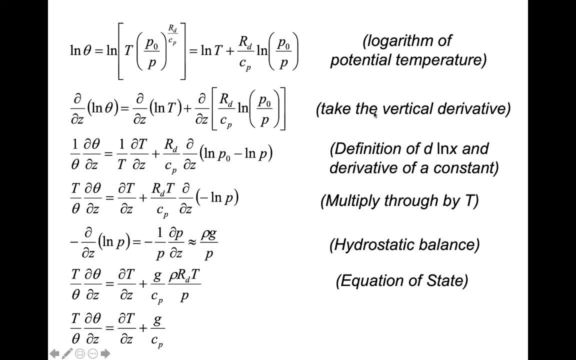 fundamental aspect of the atmosphere. We're now going to take the vertical derivative of this. so d by dz, We do d by dz on both sides. We're going to use the definition of the derivative of log x and the derivative of the constant and rewrite this equation in this form. We're going to 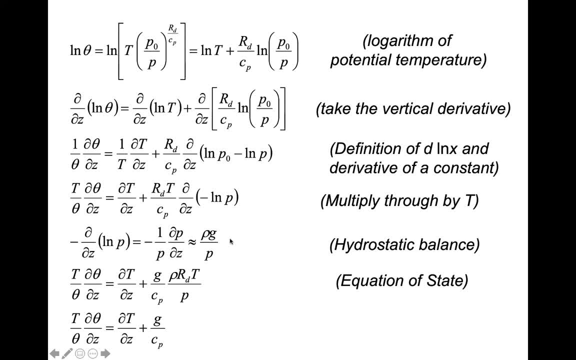 multiply through by t. We're going to use the hydrostatic balance, We're going to use the equation of state. We're going to arrive down here, at the bottom of this equation, which is at t over theta d. theta dz is equal to dt dz plus g, gravity over cp, and this is a constant. 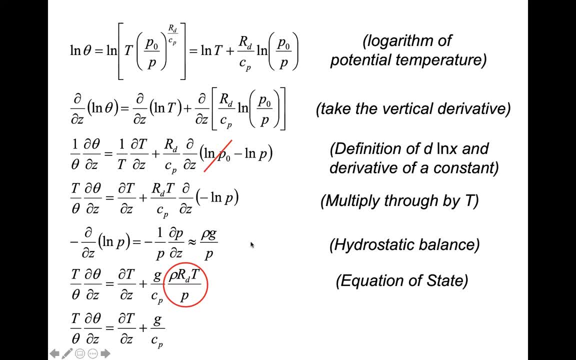 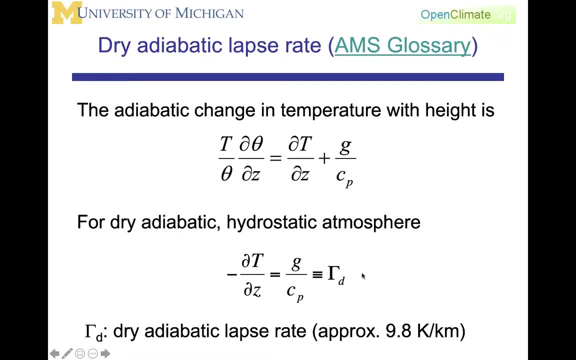 So in this derivation you see that this term goes away. You see that this term is rho RT over P. You should recognize that through the equation of state That's going to be equal to 1, and then we get to this equation here. So the dry adiabatic: 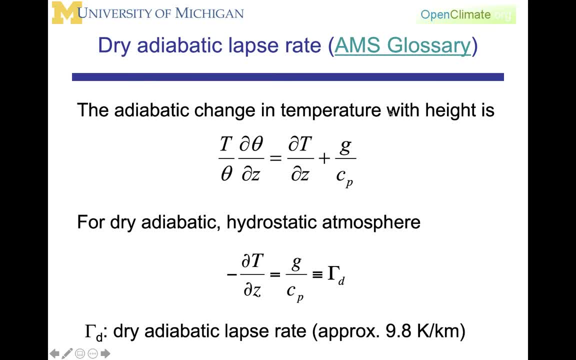 lapse rate. the adiabatic change in temperature with height is equal to this. what we just derived on the previous page. We saw that for a hydrostatic atmosphere that was dry adiabatic, that d theta dz was equal to 0. Hence dt dz is. 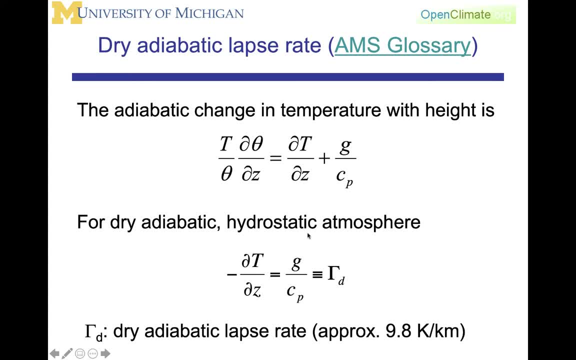 equal to minus g over Cp, and this g over Cp is called the dry adiabatic lapse rate, and that is approximately 9.8 or 10 Kelvin per kilometer In a dry atmosphere. this profile is called the dry adiabatic lapse rate, and that is approximately 9.8 or 10 Kelvin per kilometer In a dry atmosphere. this profile is 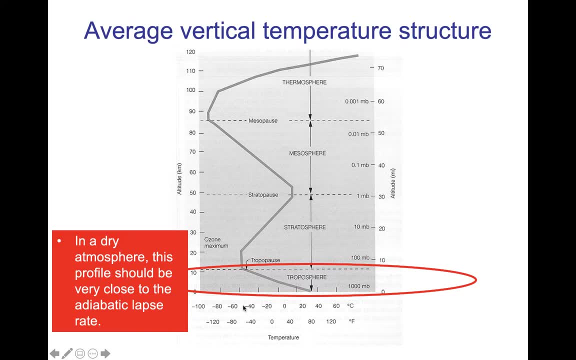 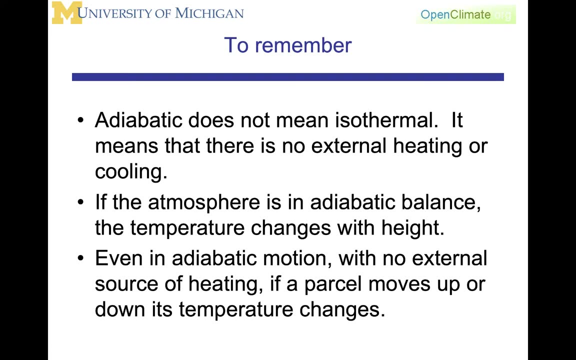 equal to 0.8 or 10 Kelvin per kilometer. In a dry atmosphere, this profile is would be very close to the dry adiabatic lapse rate. Remember adiabatic does not mean isothermal, It means there is no external heating or cooling. If the 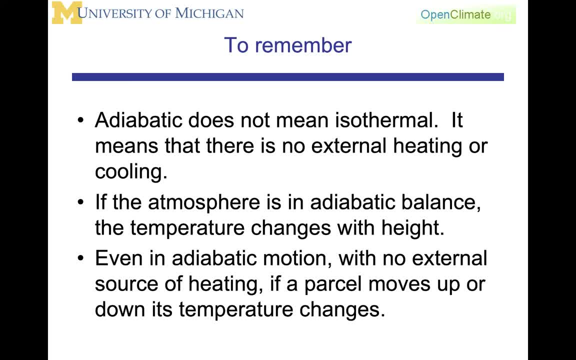 atmosphere is an adiabatic balance. the temperature changes with height, Even in adiabatic motion with no external sources of heating or cooling. If a parcel moves up or down, its temperature changes. It's worth thinking about that and then adding water. 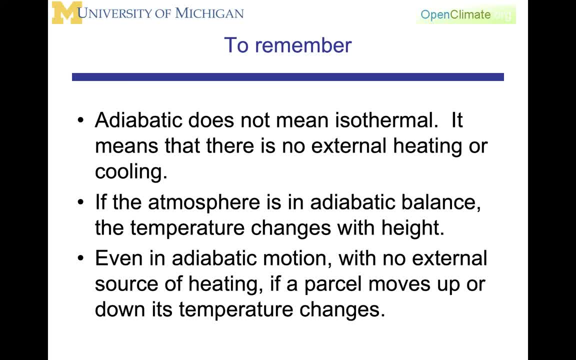 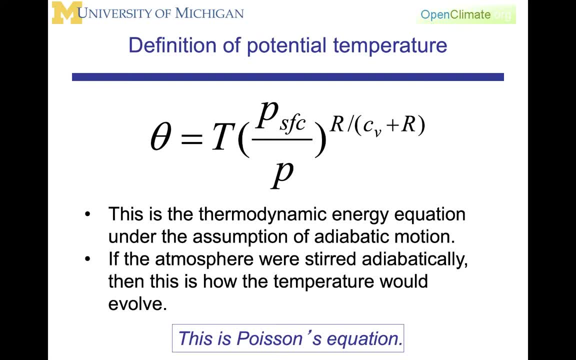 to that parcel to think about how water might change that and hence what we might call a wet adiabatic lapse rate. We use the definition of potential temperature here, and I just want to state that the potential temperature is in fact the thermodynamic energy equation, under the assumption of: 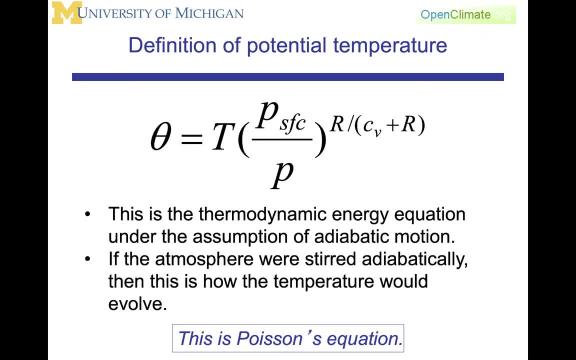 adiabatic motion. Hence, if you go back to the thermodynamic equation, make the assumption of adiabatic motion, so we take a J out- then this is what the thermodynamic equation reduces to. Hence, if the atmosphere were stirred,